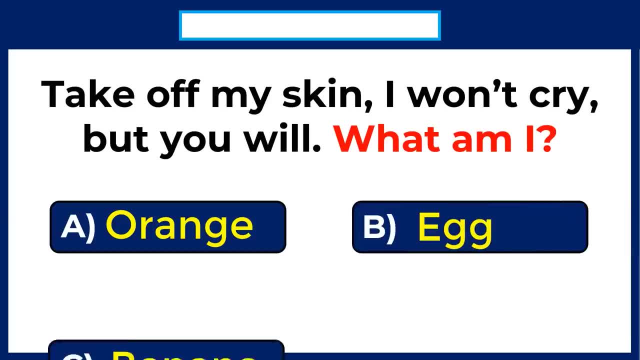 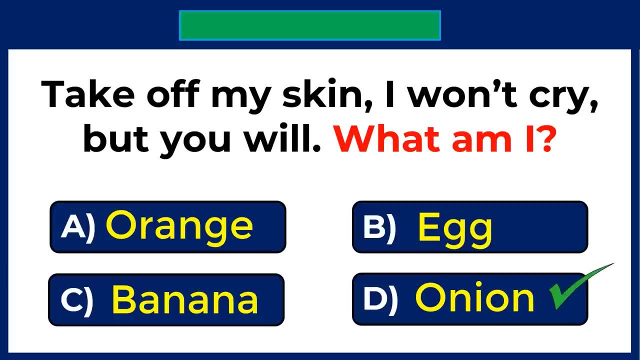 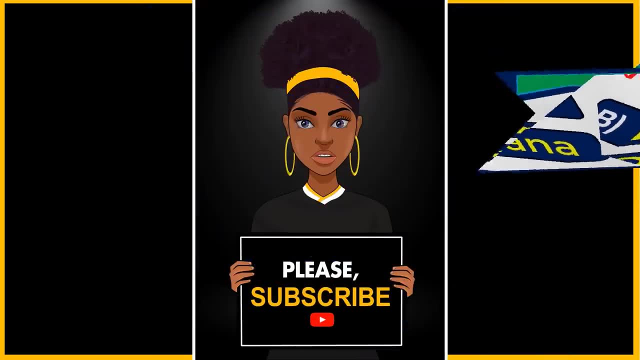 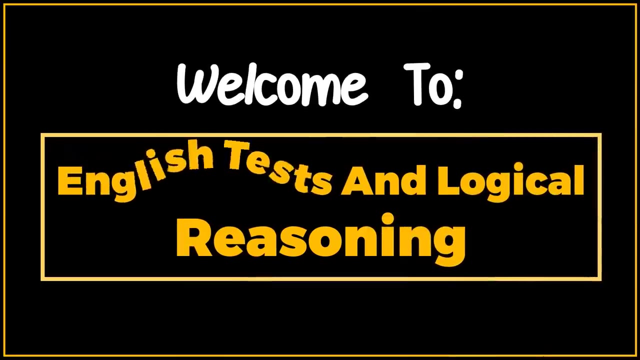 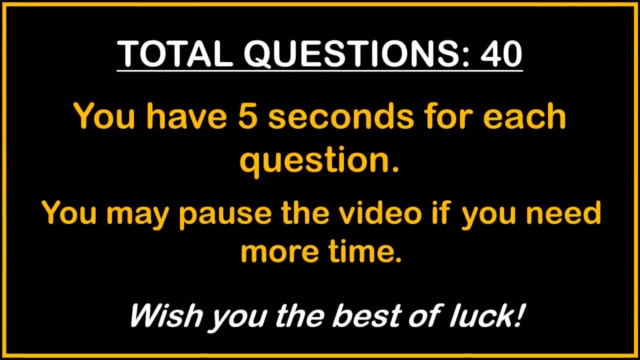 Take off my skin. I won't cry, but you will. What am I? The correct answer is option D, onion. Welcome to English Tests and Logical Reasoning. Total questions: 40.. You have 5 seconds for each question. you may pause the video if you need more time. Wish you the best of luck. 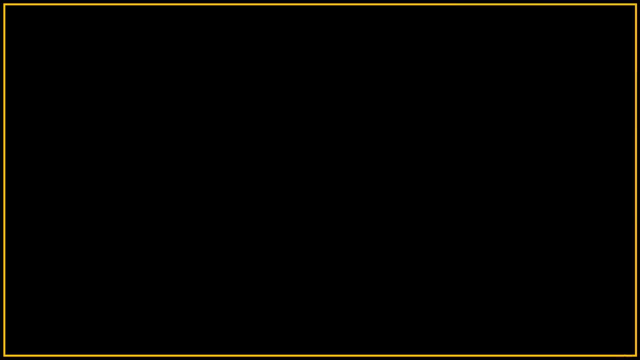 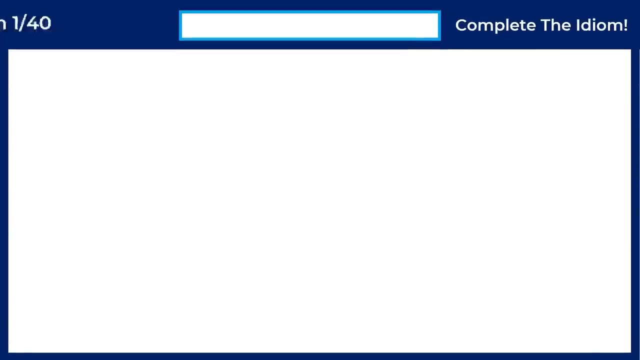 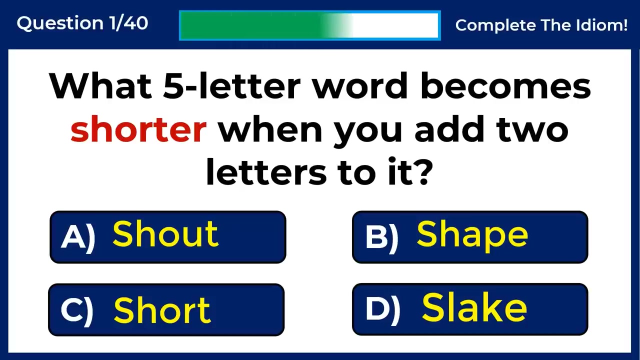 Riddles, Are you ready? Let's begin. The correct answer is option D, onion. You have 5 seconds for each question. you may pause the video if you need more time. Wish you the best of luck. Riddles, Are you ready? Let's begin. You have 5 seconds for each question. you may pause the video if you need more time. Wish you the best of luck. Riddles, Are you ready? Let's begin. You have 5 seconds for each question. you may pause the video if you need more time. Wish you the best of luck. Riddles: Are you ready? Let's begin. You have 5 seconds for each question. you may pause the video if you need more time. Wish you the best of luck. Riddles: Are you ready? Let's begin. You have 5 seconds for each question. you may pause the video if you need more time. Wish you the best of luck. 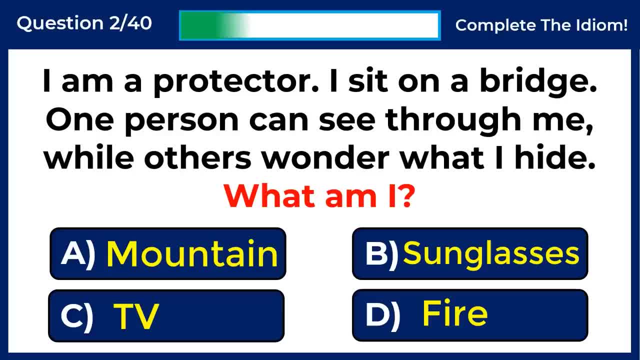 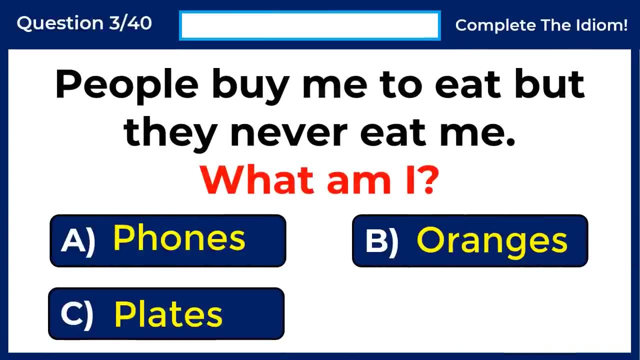 Riddles. Are you ready? Let's begin. You have 5 seconds for each question. you may pause the video if you need more time. Wish you the best of luck. Will you Place it on this teeth? will to mesa? Will you place it on this teeth? 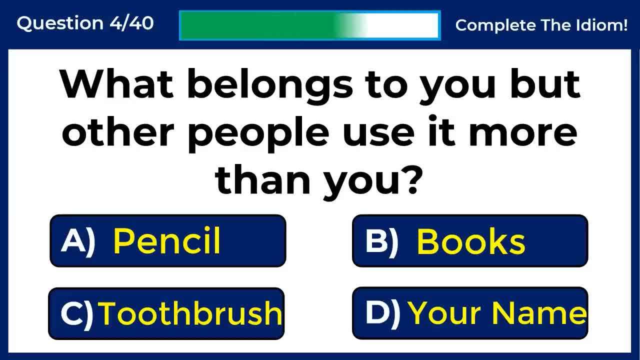 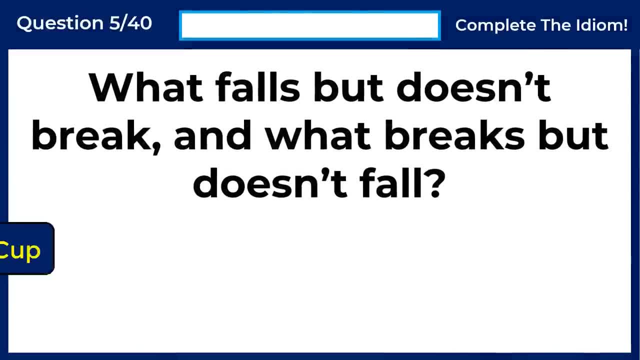 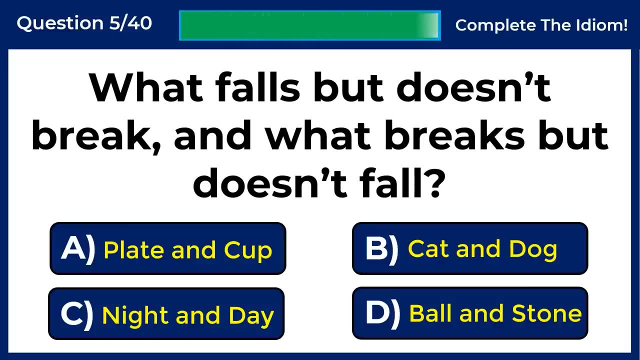 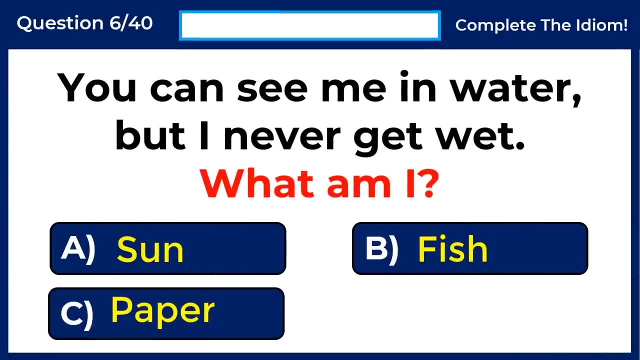 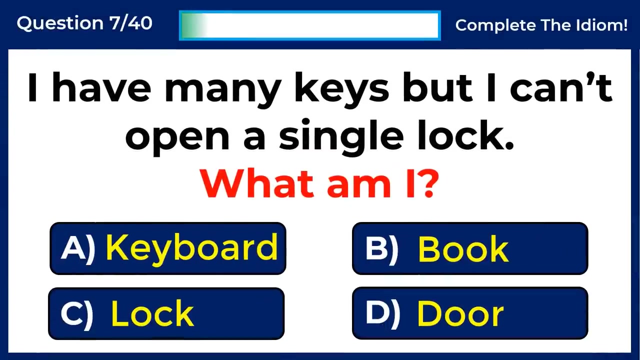 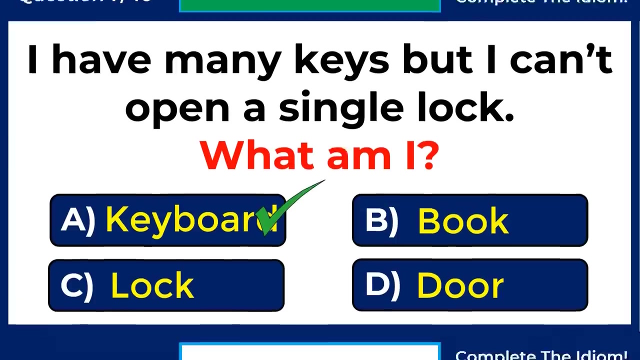 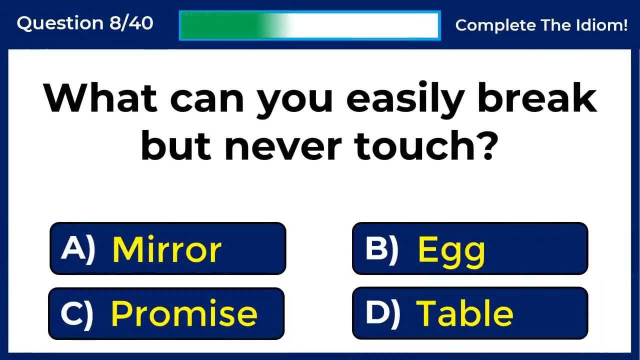 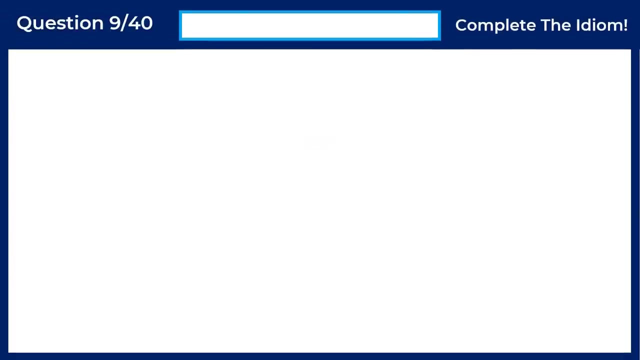 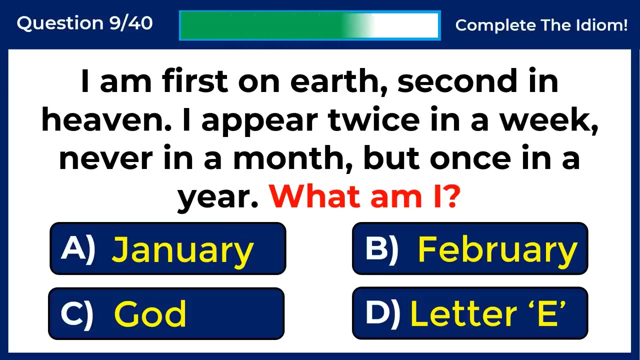 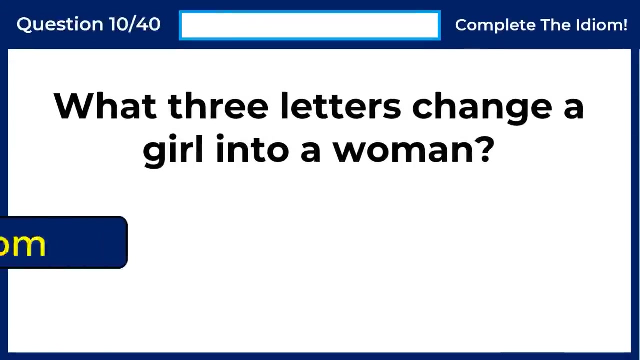 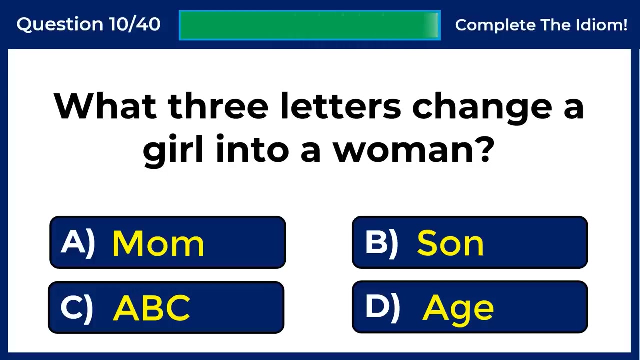 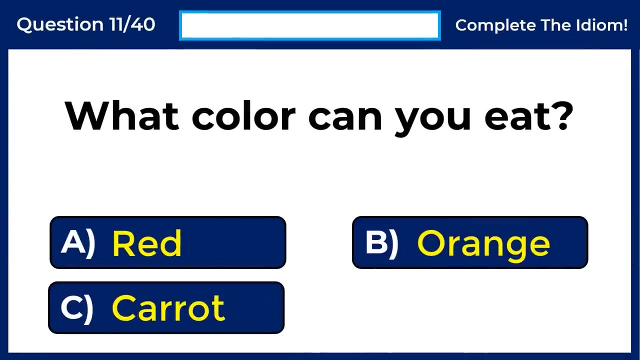 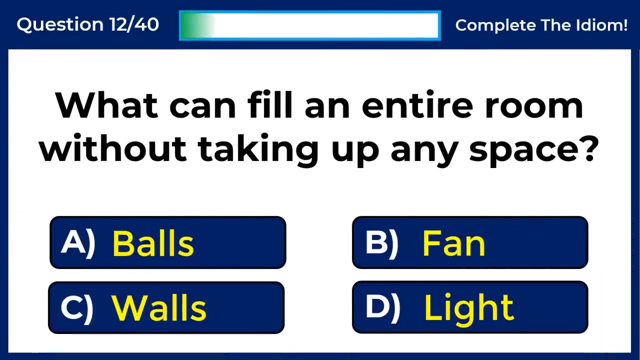 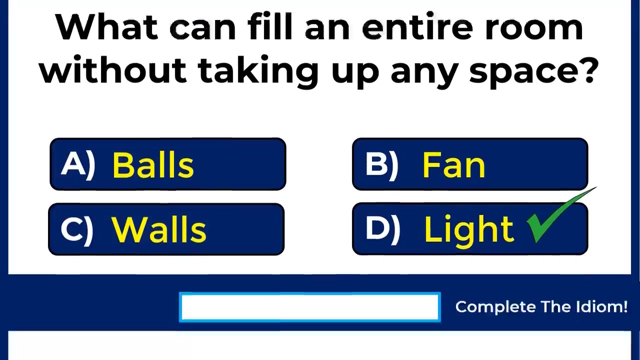 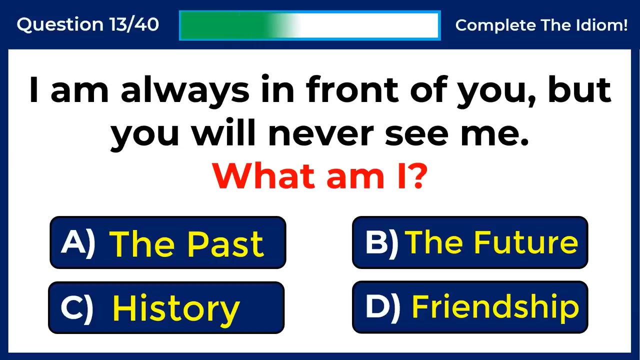